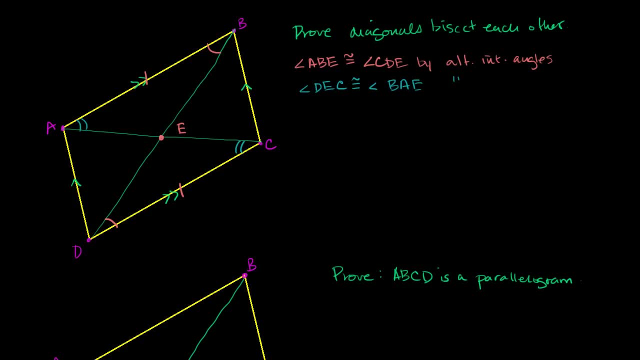 by angle side angle. So we know that triangle- I'm going to go from the blue to the orange, to the last one. Triangle ABE is congruent to triangle blue, orange and the last one, CDE. Now what does that do for us? 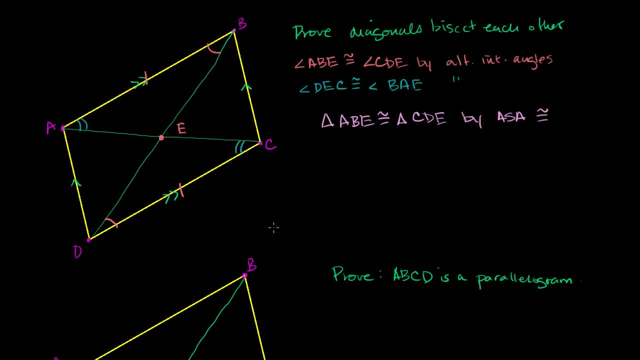 Well, we know, if two triangles are congruent, all of their corresponding features, especially all of the corresponding sides, are congruent. So we know that side EC corresponds to side EA, Or I could say side AE It corresponds to side CE. 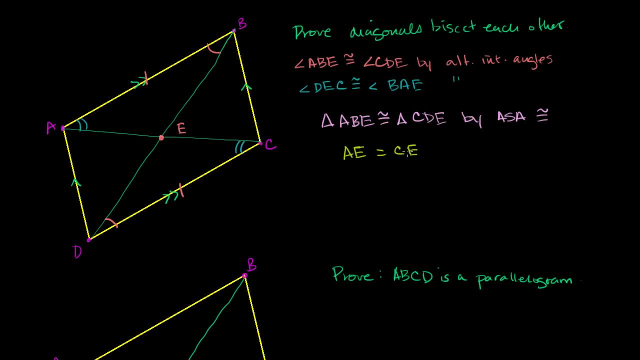 They're corresponding sides of congruent triangles, So their measures or their lengths must be the same. So AE must be equal to CE. Let me put two slashes, since I already used one slash over here. Now, by the same exact logic. we know that DE, we know that. 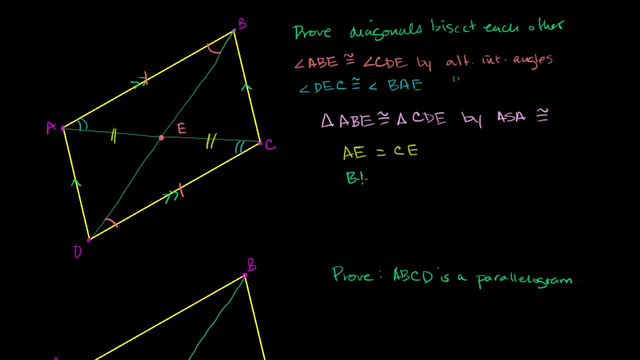 let me focus on this. we know that BE must be equal to DE Once again. So they're corresponding sides of two congruent triangles, So they must have the same length. So this is corresponding sides of congruent triangles. So BE is equal to DE. 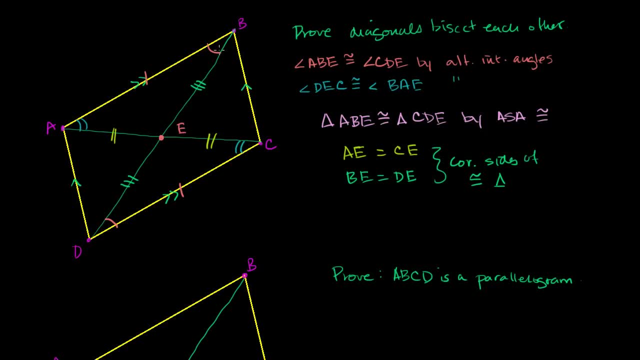 And we've done our proof. We've shown that look diagonal. DB is splitting AC into two segments of equal length and vice versa, AC is putting DB into two segments of equal length, So they are bisecting each other. Now let's go the other way around. 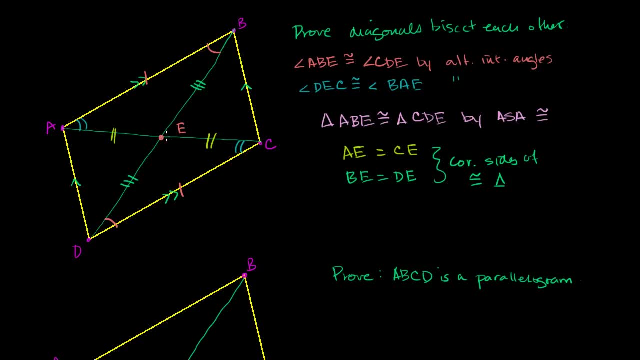 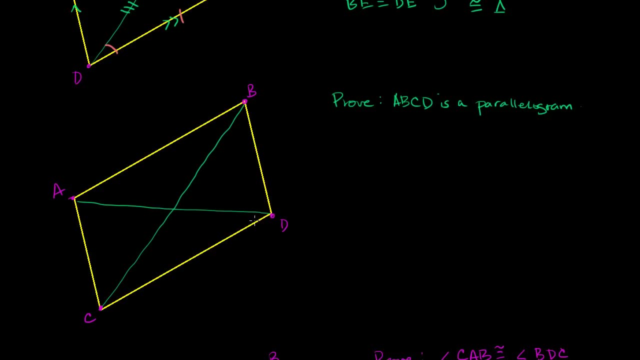 Let's prove to ourselves that if we have two diagonals of a quadrilateral that are bisecting each other, that we are dealing with a parallelogram. So let me see. So we're going to assume that the two diagonals are bisecting. 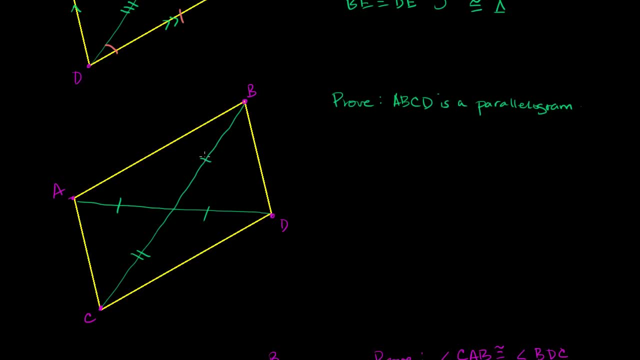 each other. So we're assuming that that is equal to that And that that right over there is equal to that. Given that, we want to prove that this is a parallelogram, And to do that we just have to remind ourselves. we just 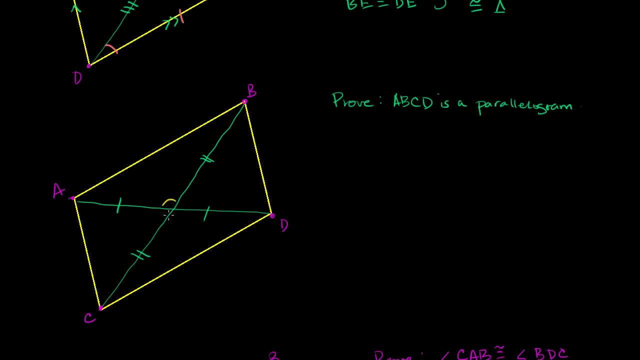 have to. We have to remind ourselves that this angle is going to be equal to that angle. It's one of the first things we learn, because they are vertical angles. So let me write this down: C. let me label this point: CED, angle CED. 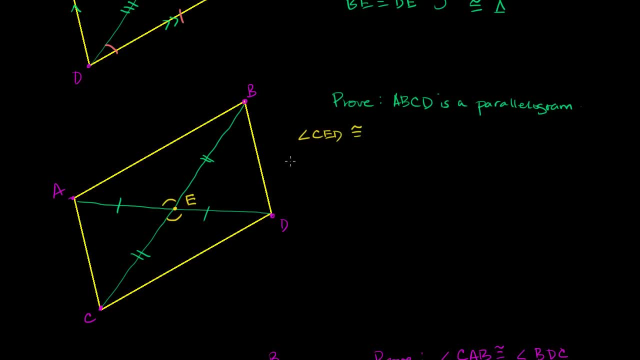 is going to be equal to, or is congruent to, angle. So I start at: C is BEA, Angle, BEA And that? what is that? Well, that shows us that these two triangles are congruent because we have a corresponding size. that are congruent. 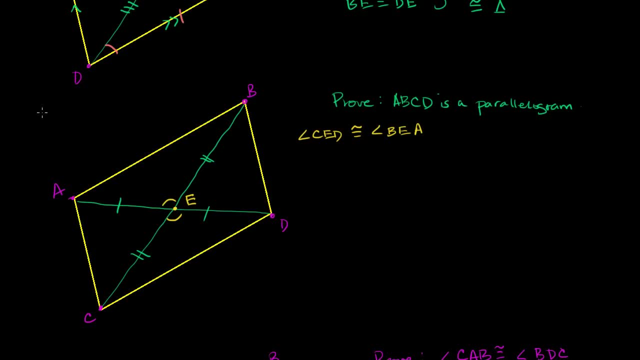 an angle in between and then another side. So we now know that the triangle- I'll keep this in yellow- triangle- AEB is congruent to triangle DEC by side, angle side congruency. By SAS: congruent, Congruent triangles. 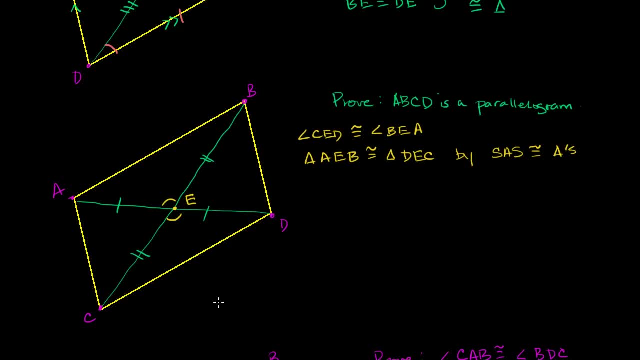 Fair enough. Now, if we know that two triangles are congruent, we know that all of the corresponding sides and angles are congruent. So, for example, we know that angle CDE is going to be congruent to angle. You can see: CDE is going to be congruent to BAE. 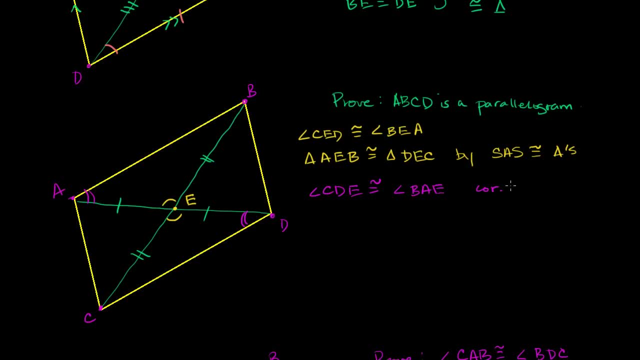 And this is just Corresponding angles of congruent triangles. And now we have this transversal or this kind of transversal of these two lines that could be parallel if the alternate interior angles are congruent, And we see that they are. 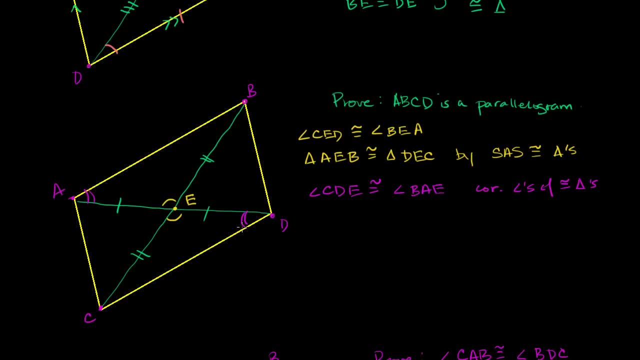 These two are kind of candidate alternate interior angles And they are congruent. So AB must be parallel to CDE. So AB- which I'll just draw one arrow- AB must be parallel to CDE. AB is parallel to CDE by alternate interior angles. 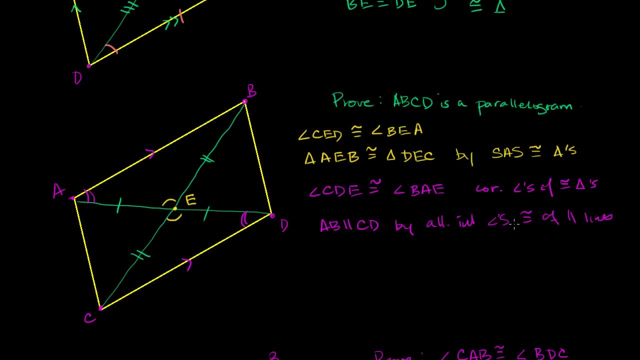 congruent of parallel lines. I'm just writing in some shorthand- Forgive the cryptic nature of it, although I'm saying it out- And so we can then do the exact same logic. We've just shown that these two sides are parallel. 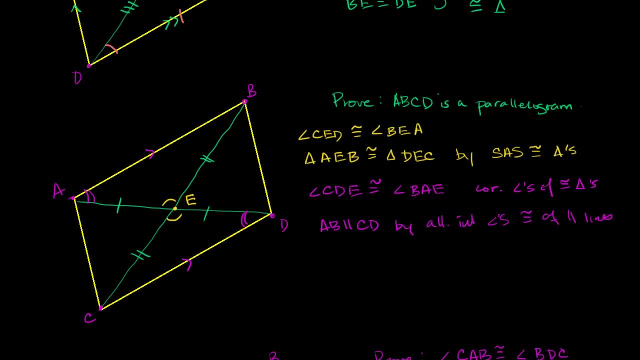 We can then do the exact same logic to show that these two sides are parallel, And I won't necessarily write it all out, But it's the exact same proof to show that these two. So first of all, we know that this angle.